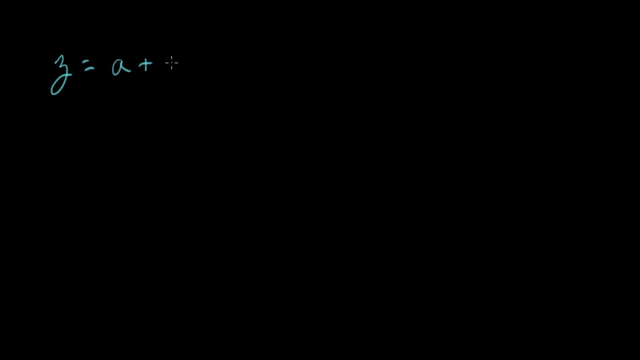 and we'll say it's made of two parts: a real part called a and an imaginary part called b. So now what I wanna do is what happens if we multiply z by j, one time J times z, and that equals j times a plus jb. 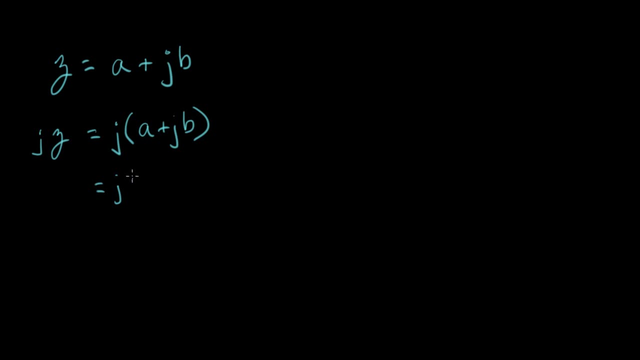 and let's just multiply it through equals j times a plus j times j times b. A and b have now switched places, so we're gonna put j a on this side, j a on this side, and what do we have here? 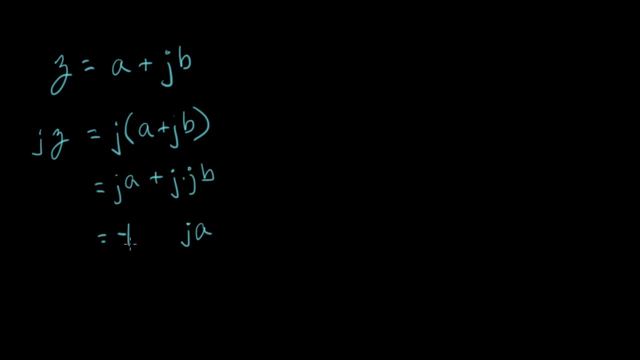 J times. j is minus one, so we have minus b plus j a. So now we have expressions for z and jz and I wanna go plot these on a complex plane and see what they look like. And here's the real axis, here's the imaginary axis. 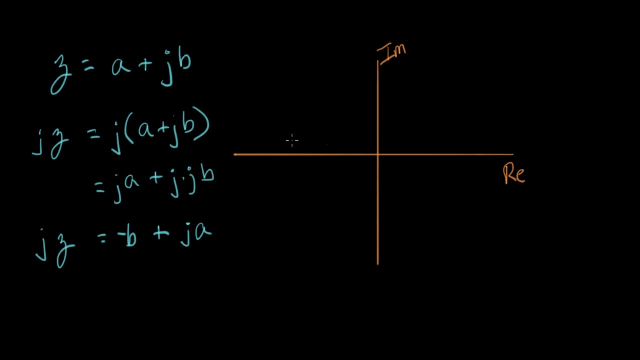 And let's first plot. let's plot z. let's say z has a large real value and that would be a. and let's say that b is a smaller value. we'll put b here And that means that z is at a location. 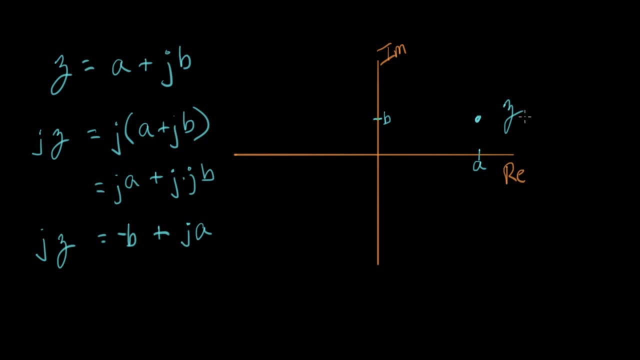 in the complex plane right there, If we can plot the dotted lines. If we can plot the dotted lines, That's z in the complex plane. So now let's put jz on the same plot. jz has a real component of minus b. 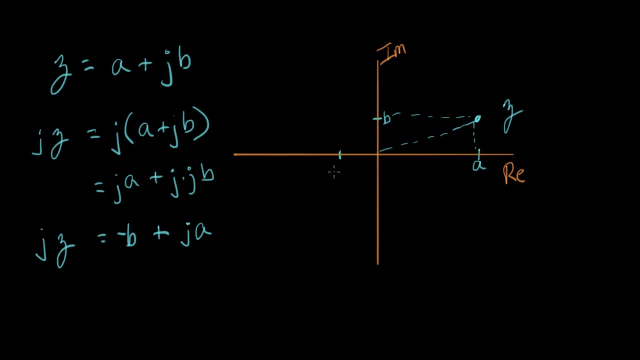 so that would be right about here. Here's minus b, and it has a imaginary component of plus a, So let's swing a. a goes all the way up to about here, And so that's the location of jz. And let me draw the hypotenuse of that. 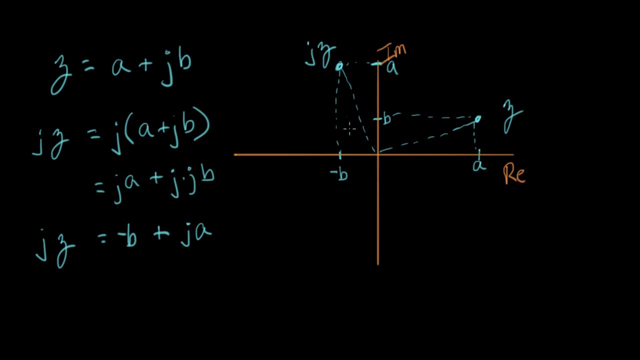 This is the vector representing jz right there. So now we have a bunch of triangles on the page, and what I wanna demonstrate is that this angle right here is 90 degrees. So one way to do that. let's see if we can do that. 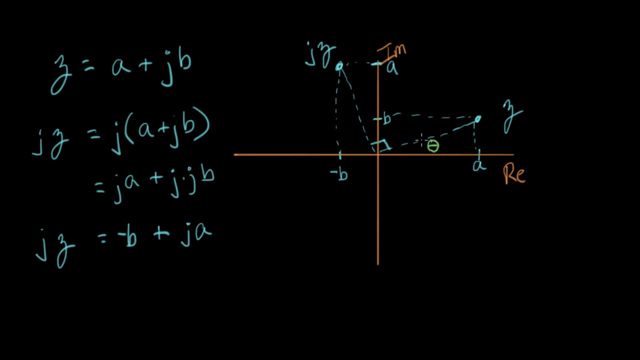 Let's say, this angle here is theta. That's the angle right there. Now, this triangle here, this triangle that we've sketched in. just imagine in your head that we're gonna rotate that angle up until the a leg of that triangle. 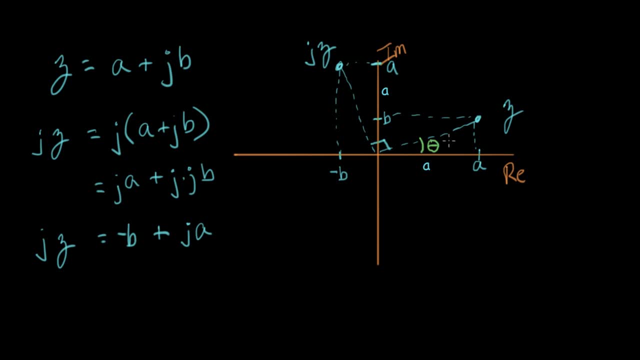 is resting right here on the imaginary axis. So this triangle rotates up to become this triangle here. Since we've moved that triangle, we know that this angle here that's also theta. It's the same triangle just rotated up. And what does that make this angle here? 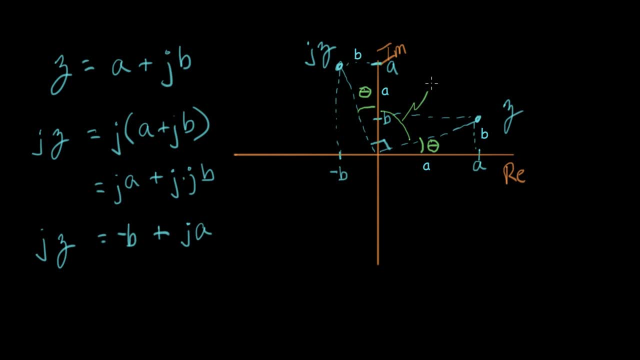 This angle here that equals 90 degrees minus theta. So if I combine this theta angle with this angle here, what do I get? I get theta plus 90 degrees minus theta and we get 90 degrees. So we just showed that this angle right here. 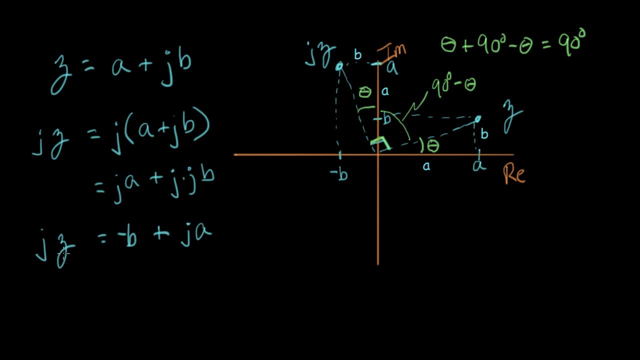 is a 90 degree angle. That demonstrates that any complex number z, if I multiply it by j, that results in a positive rotation of 90 degrees. So let's do this rotation again, only this time instead of using the rectangular coordinate. 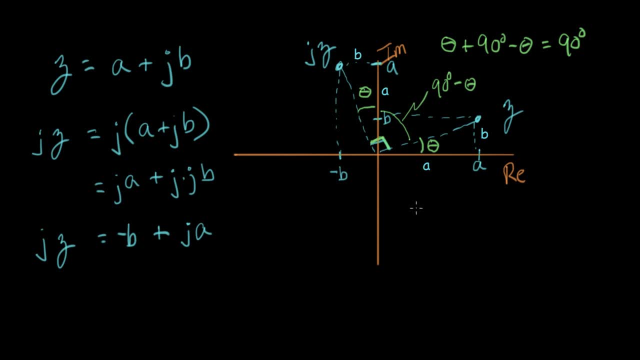 system, let's use the exponential representation. So in the exponential notation we say in general, z equals some radius times e to the j theta, where this is the angle theta and r is the length of this hypotenuse here to get out to z. 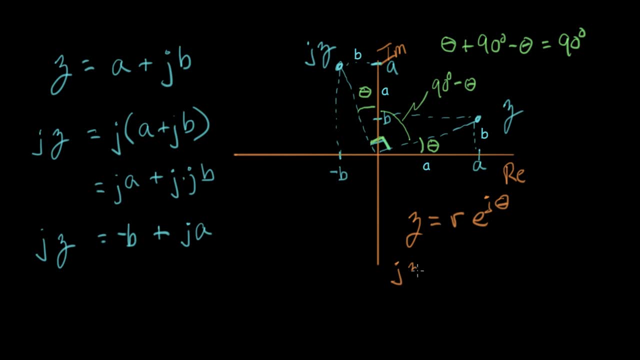 So what is in this notation? what is jz? And that equals j times, r e to the j theta. So now I'm gonna do a little trick where I'm gonna represent j in exponential notation. So if I color in dark here, this is j. 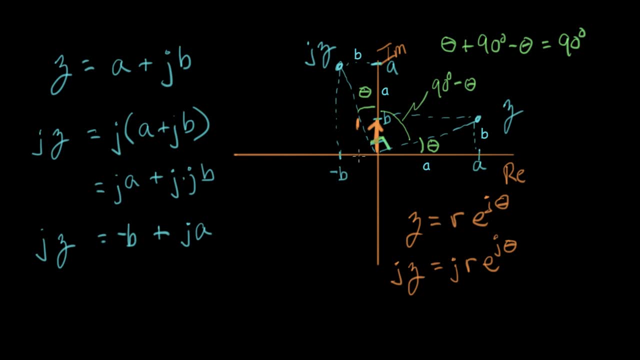 The vector j is right there and it has a magnitude of one and it points straight up on the imaginary axis. So I can represent j like this. I can say j is e to the j 90 degrees. That's equivalent to this j here.